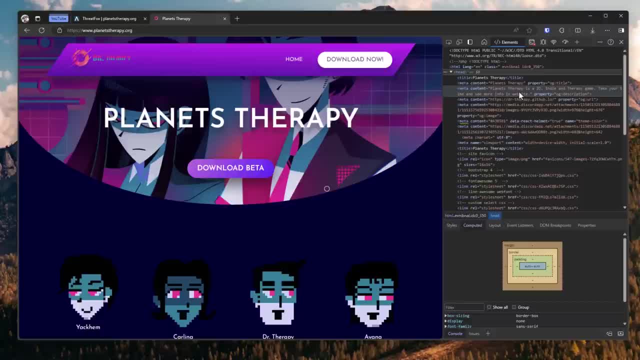 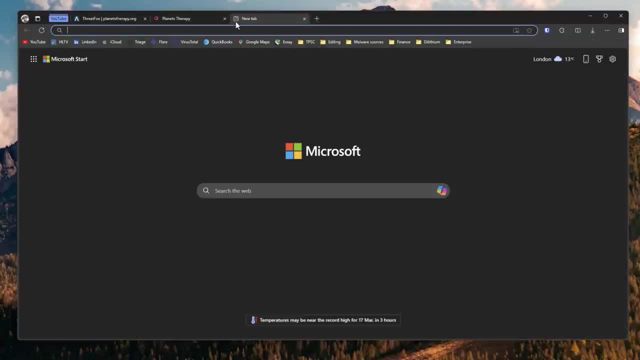 And if we expand the head, as you can see, we've got the description, we've got a reference to GitHub and we've also got some references to Discord. But not everyone can understand HTML. But what you can do is you can always use websites like ScamAdvisor and simply look up. 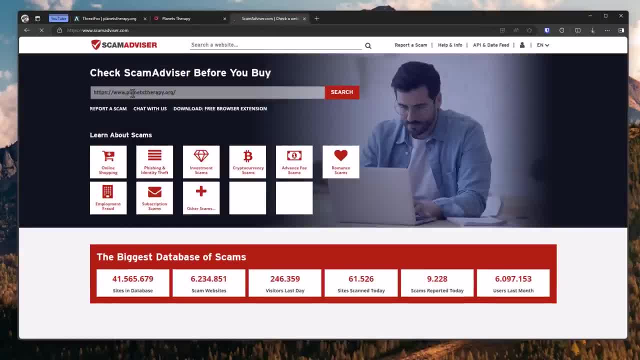 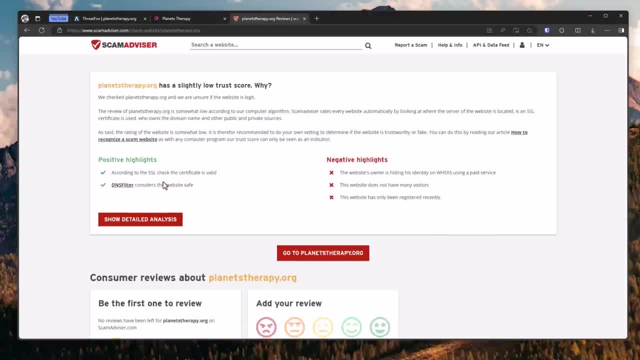 whatever website you're visiting. So let's say we wanted to do a deeper dive into planistherapyorg. It has a trust score of 56. So if we scroll down, it's got a valid SSL certificate which we can also check from here with the nice lock. But it's also got a paid service to hide its identity. Now 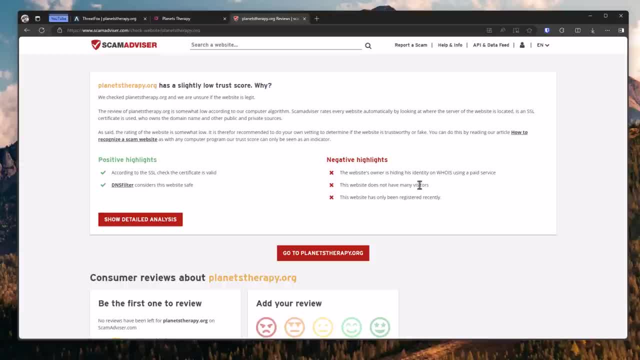 this is not uncommon- A lot of websites do that- but it also doesn't have many, and it's only been registered very recently. Now, this is all data that's publicly available through the ICANN record. Now, on the contrary, if we search for a website like the pcsecuritychannelcom. 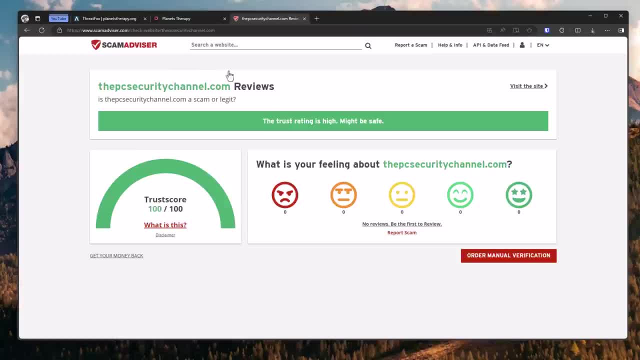 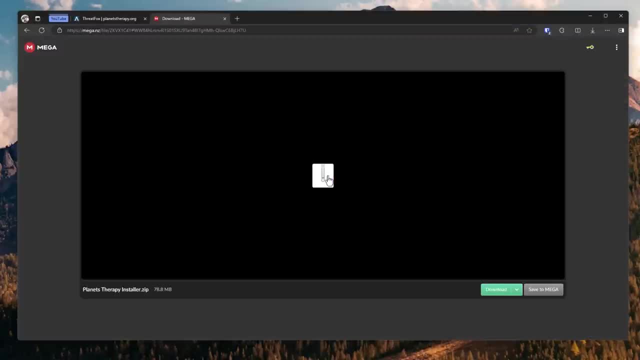 you're going to see instantly that we have a trust score of 100. So you know you can safely visit us. Next, against our judgment, we're actually going to download the malware, which brings us to malware analysis. There was a time when malware analysis was really difficult and you would need 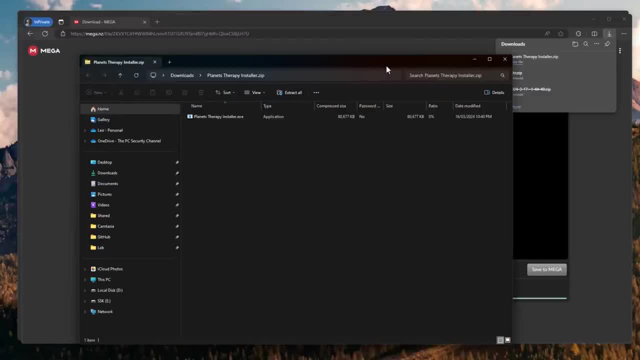 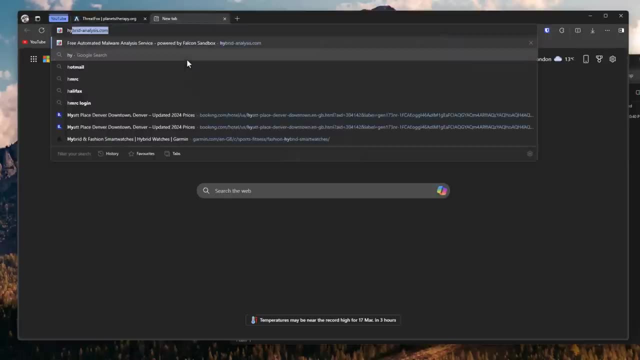 an expert in bytecode, But now we're going to do a deeper dive into planistherapyorg. So once we extract this belligerent exe, put it on our desktop, we can analyze it quite easily by simply going to a site like hybrid analysis, picking an operating system that we're running. 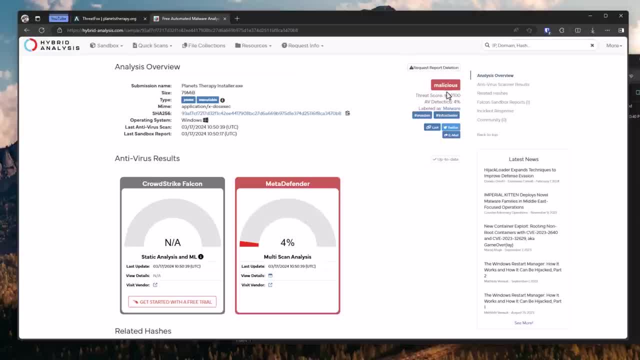 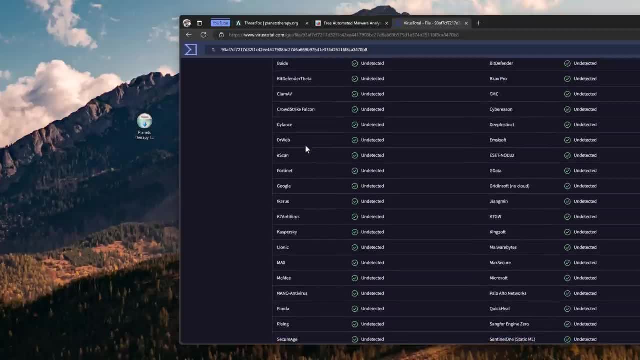 and generate a public report And within a few seconds we get a verdict that this is indeed malicious. Now you could use a variety of services, including varstotal, But, as you can see, it's not always a reliable indicator of whether or not a file is malicious. if you're just 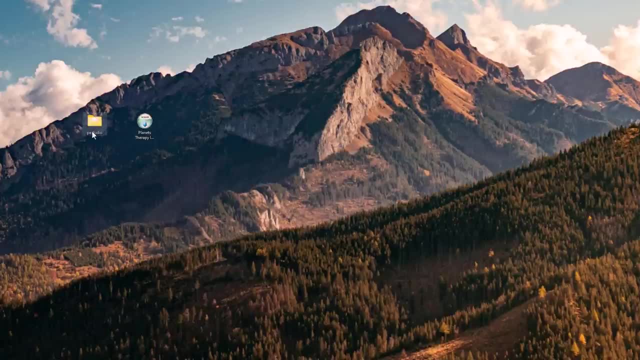 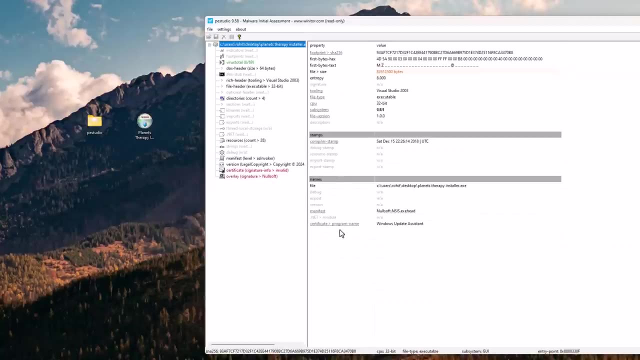 relying on the detections. But you could also skip the online services and use something like PE Studio. Drag and drop the file there and look for things in red, basically Things like the program name being Windows Update Assistant, an invalid certificate and an overlay on the exe. 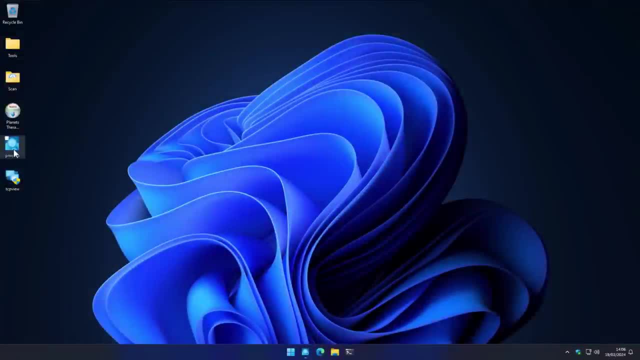 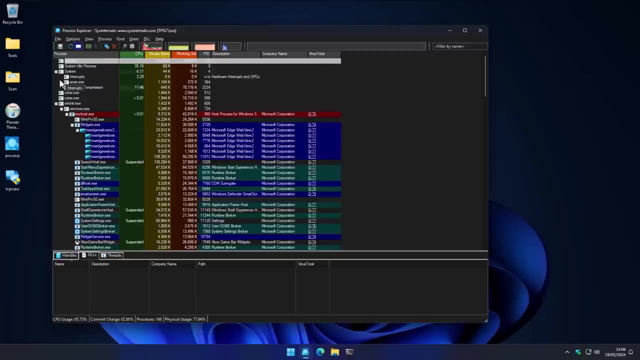 might be suspicious. The next skill I'm going to talk about is forensics, which is the ability to take a deeper look at what's happening inside a system. You don't have to use advanced tools like volatility, but everyone can download it. So let's get started. 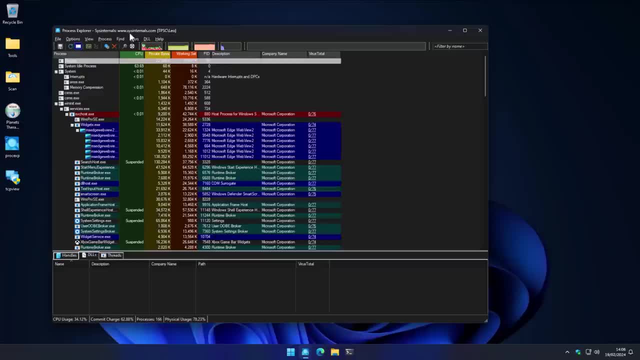 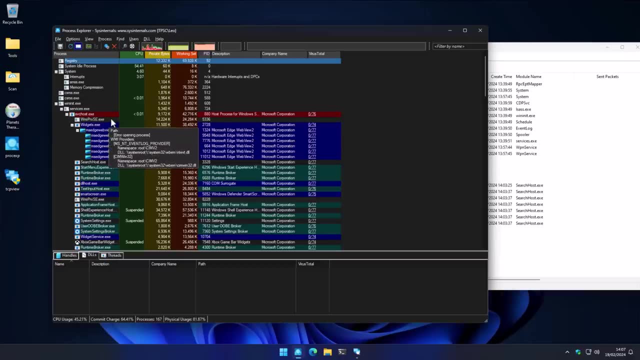 Microsoft's sysinternals suite from sysinternalscom and learn to use a couple of basic tools like Process Explorer and TCP View. Process Explorer is going to show you everything that's executing on your system: all of the processes, all of the DLLs, everything that's loaded. 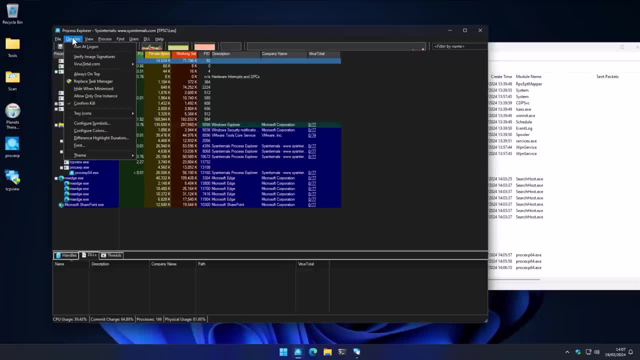 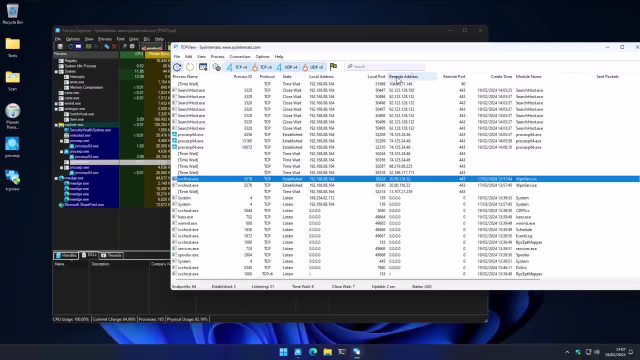 along with scan results and varstotal, if you select it in options. TCP View, on the other hand, is going to show you every connection that your computer is making to a remote address And, using the first skill investigation, you can actually figure out what's happening inside a system. 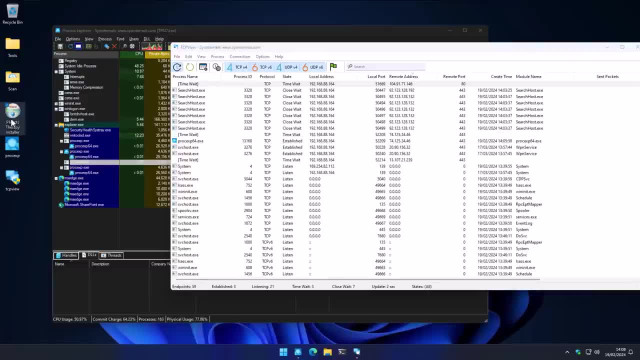 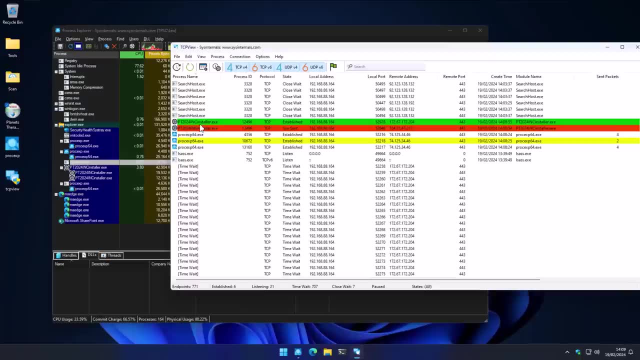 So, for instance, if we now run this file that we got from the website and it's running all of these different command line tools and we can see that this particular process that we just launched has established a connection with this IP address, It's not really showing us any UI, but it's. 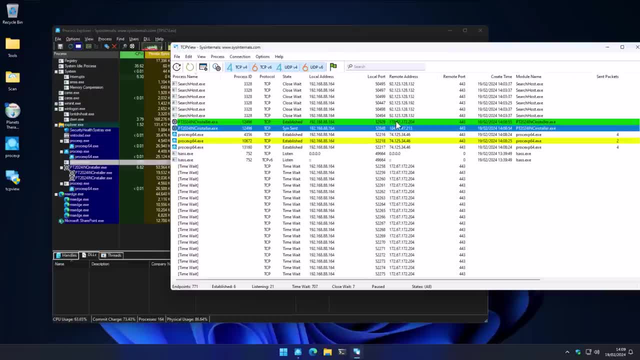 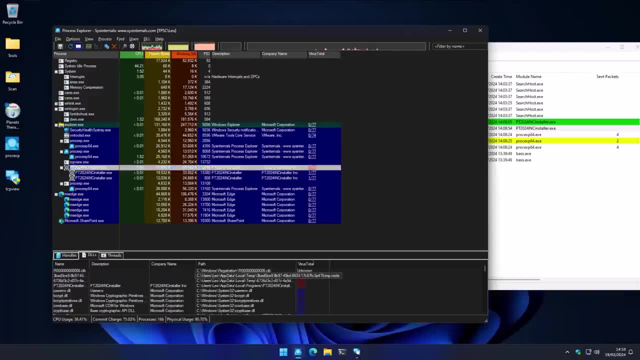 connecting and communicating with a remote address, which suggests some kind of Trojan behavior. Similarly, this particular process is loading a lot of DLLs, some of which are being detected. Views like this can load a lot of DLLs and some of them are being detected. So if you're using 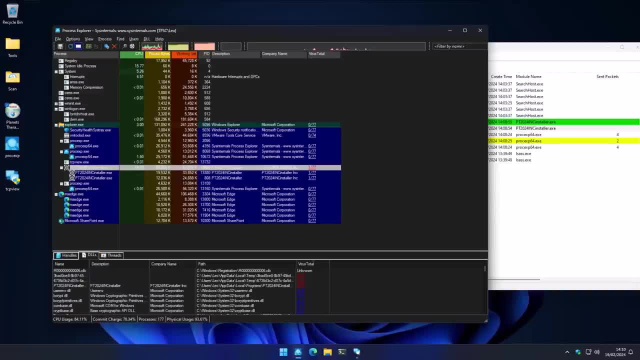 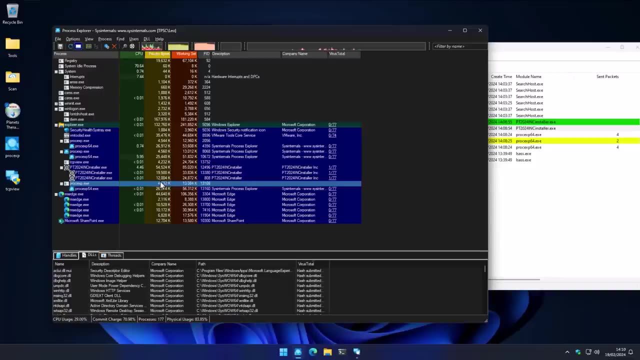 the process name, you can read the description and over time you're going to familiarize yourself with what runs on your system by default, so that when you run something new you're going to be able to spot it instantly. As time goes on, I think the basic skills of being able to investigate 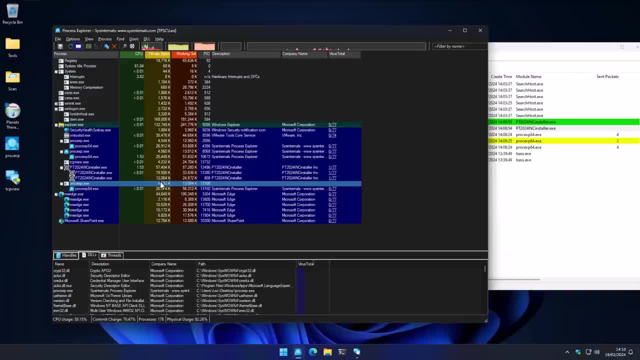 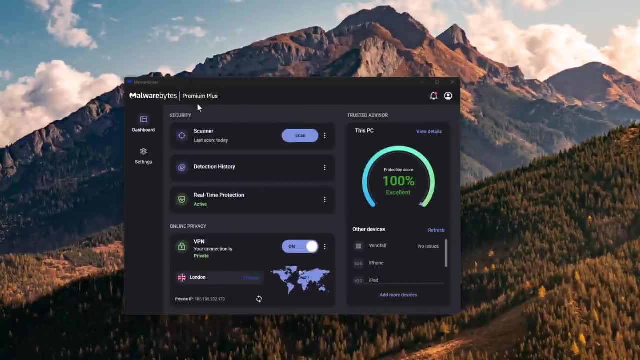 and verify what you're looking at are going to be more and more important Now. I hope you found this video helpful. Please like and share it, if you did Now. this video is sponsored by one of my favorite cybersecurity tools, which is Malwarebytes, a full-fledged lightweight. 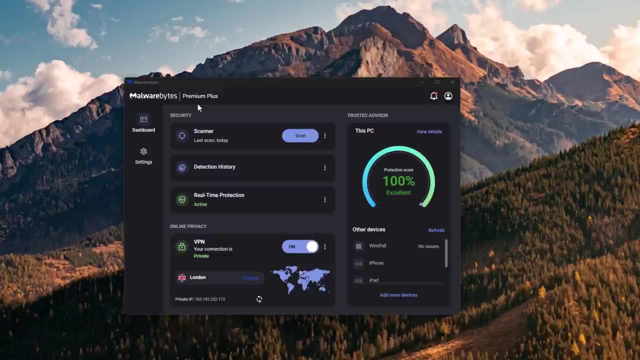 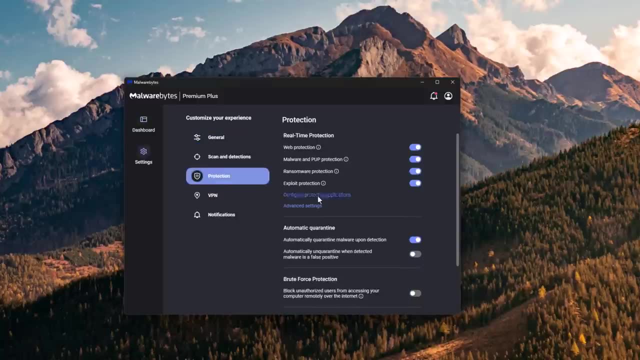 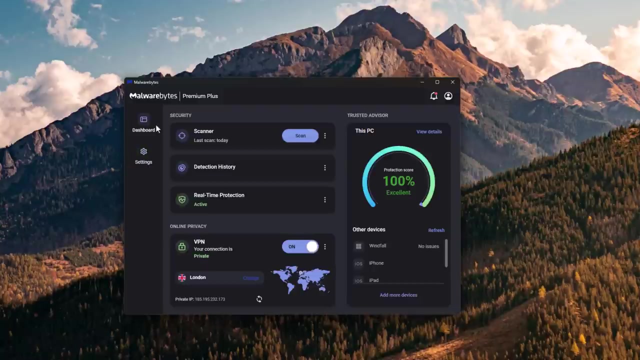 antivirus program that has routinely demonstrated good detection capabilities in our tests, as well as massively improved their UI recently, And if we look at settings, it has everything from ransomware and exploit protection to the ability to block pen testing attempts. Many of you may have heard of Malwarebytes as a second opinion scanner, something you 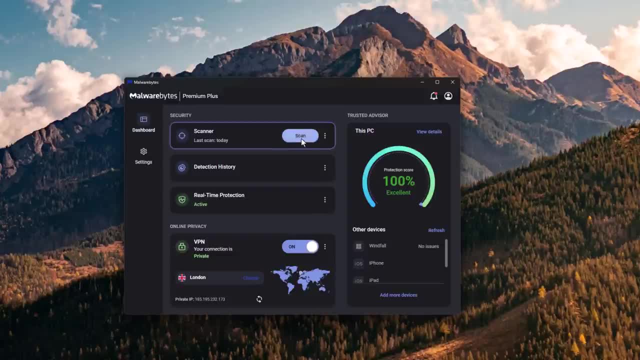 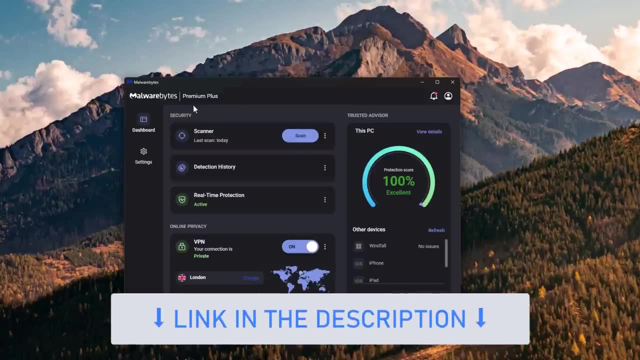 use to remove malware if your system is infected, But the brand new Malwarebytes is actually a full-on AV replacement and stops malware in real time. They recently updated their user interface. As you can see, it looks very slick in dark mode. We've done independent.